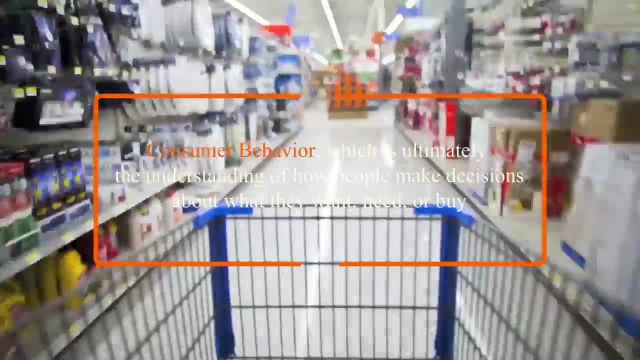 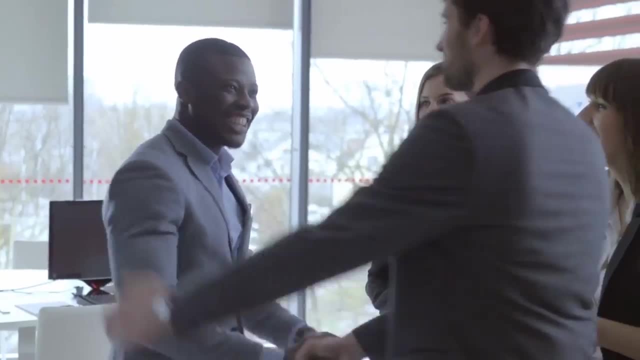 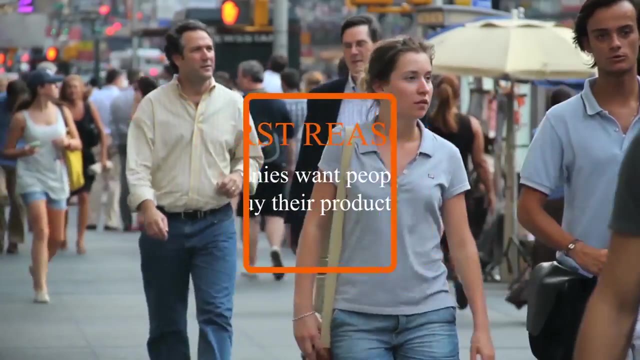 which is ultimately the understanding of how people make decisions about what they want, need or buy. The study of consumer behavior is critical for two reasons. The first reason is that companies want people, not robots, to buy their products or services. To make that happen, companies must understand people at their deepest level of need. 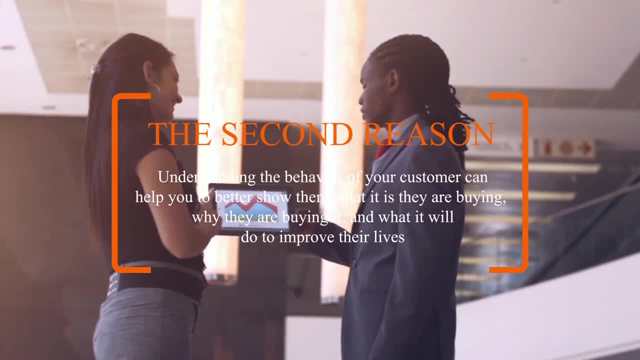 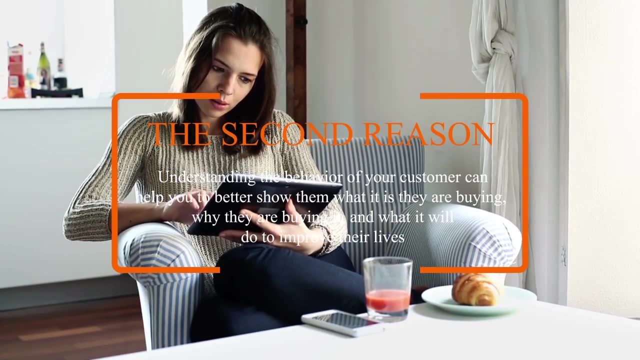 The second reason may not be so obvious. Understanding the behavior of your customer can help you better. show them what it is they're buying, why they're buying it and what it will do to improve their lives. Once you discover this, you will have a much 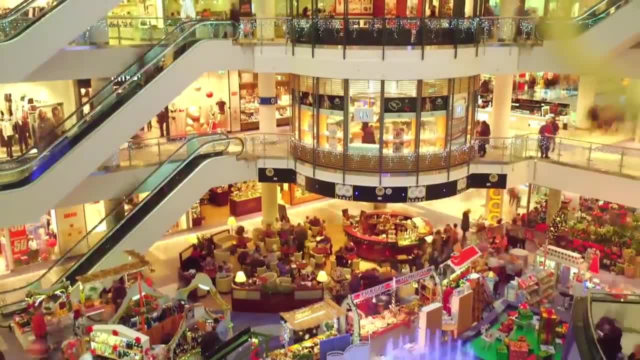 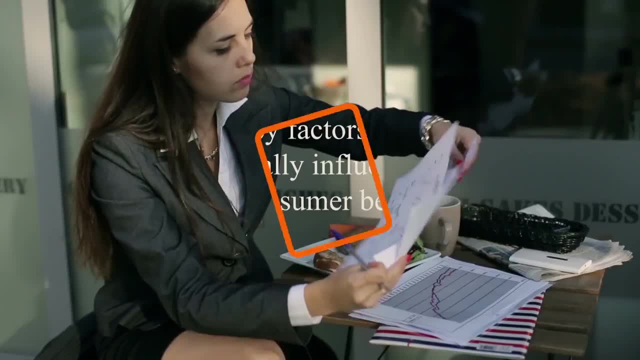 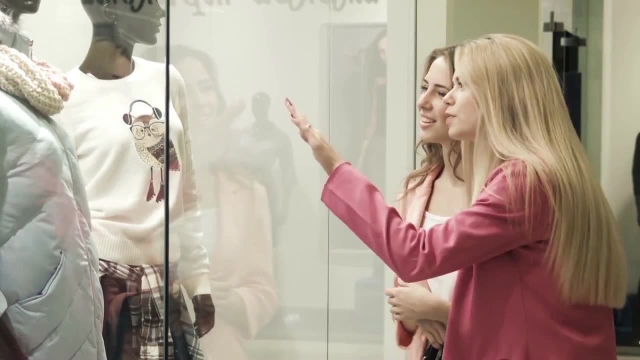 better chance at marketing your products and services to the right audience at the right time. According to iResearch Services, there are four key factors that can really influence consumer behavior. Number one is that consumer behavior is influenced by the opinion of the consumer, which can be a dominant influencing factor, Although ads affect these opinions to some. 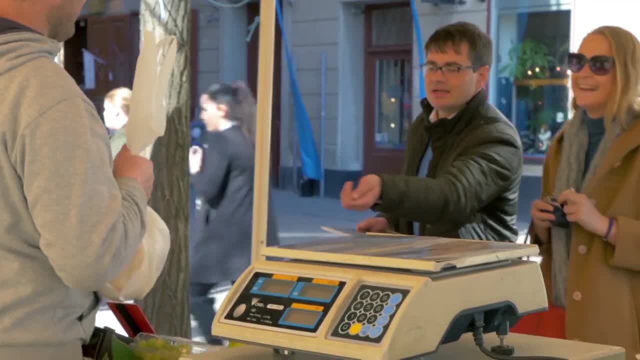 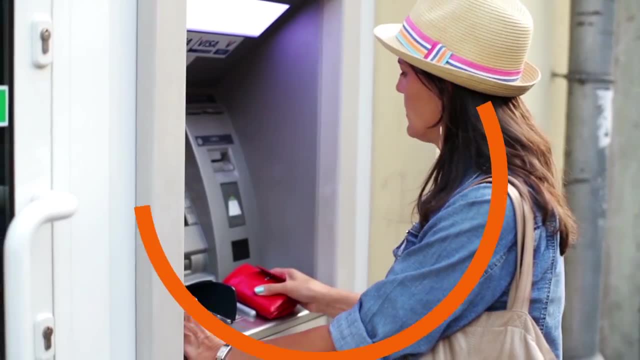 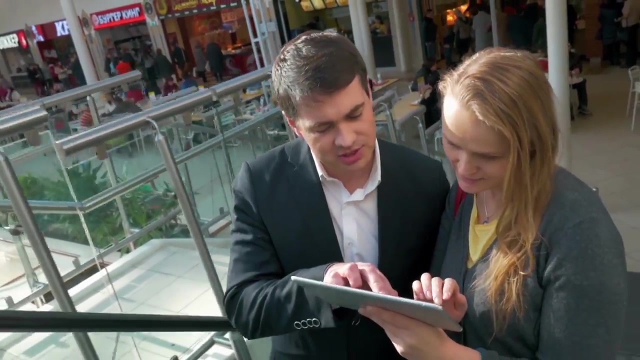 extent the personal likes and dislikes of consumers hold the greatest influence over the end purchases. The second factor is that consumer spending decisions are often influenced by economic situations. A positive economic environment can make the consumer's decisions more confident and willing to indulge in purchases than in a negative one. 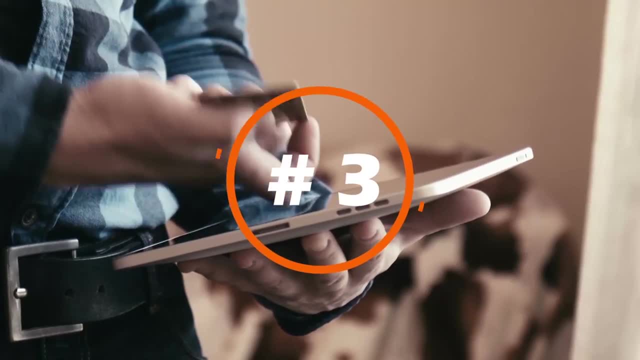 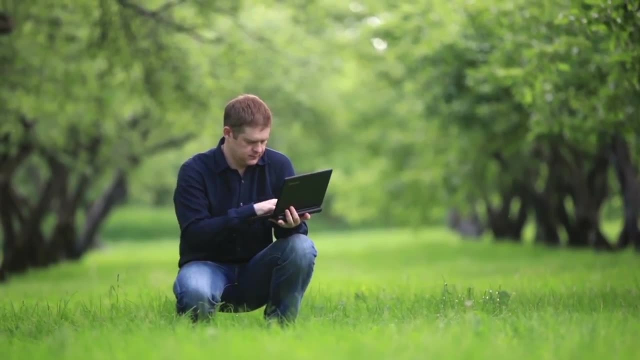 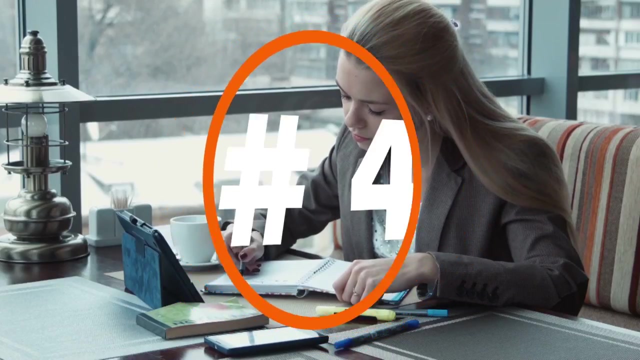 The third factor is that advertising plays a major role in influencing the purchasing decisions of consumers. Most consumers get their information from social media, So if you want to market in the modern age, you must develop a strong social media presence. The fourth and final factor is that the purchasing power of a consumer helps to influence a consumer's behavior. 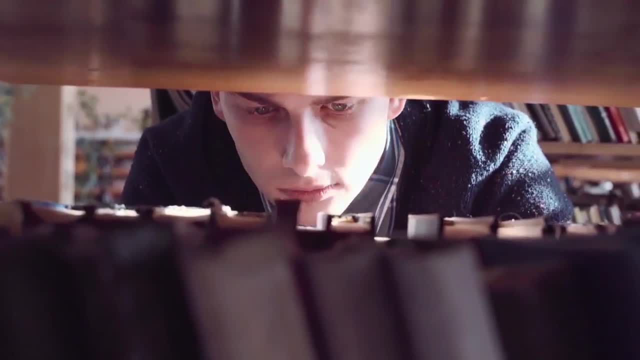 Although your product may be of high quality, if it fails to protect the consumer's behavior- it may also affect the consumer's personal taste and need- and action to meet your target buyer's purchasing ability, the sales of that product will be effective. 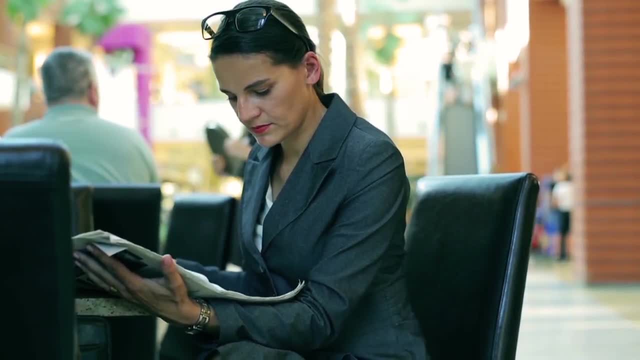 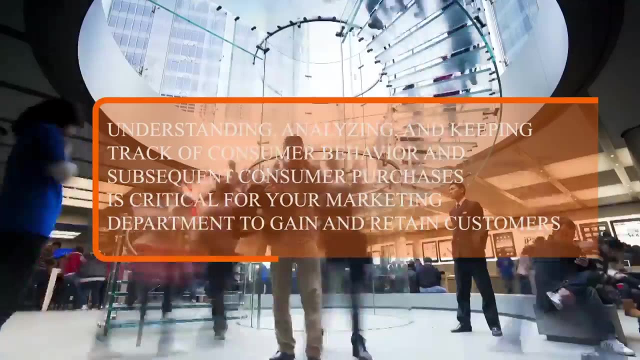 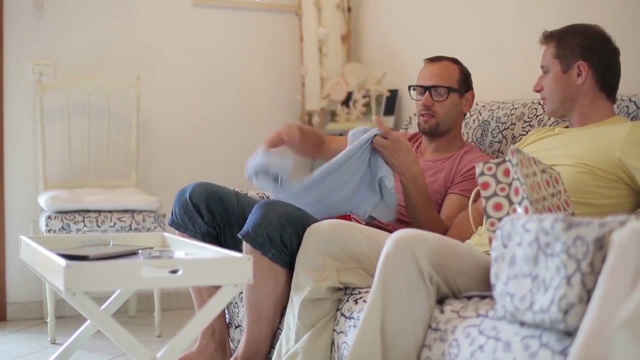 Consumer behavior is social, personal and psychological. Understanding, analyzing and keeping track of consumer behavior and subsequent consumer purchases is critical for your marketing department to gain and retain customers. It has been said that the customer is always right In the case of their behaviors and actions. this belief has never failed to give.